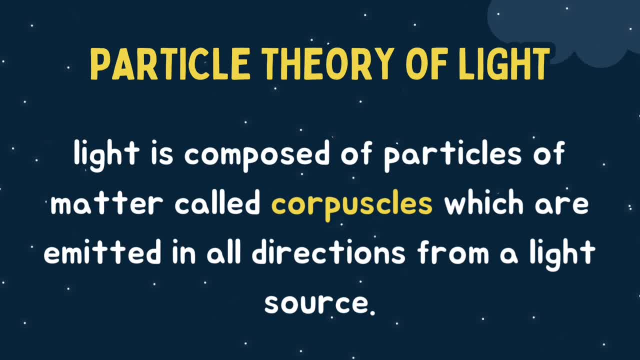 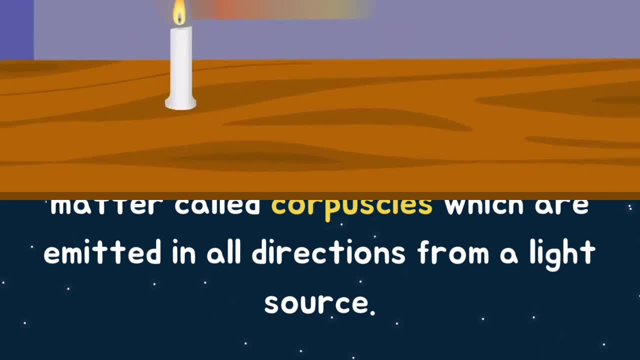 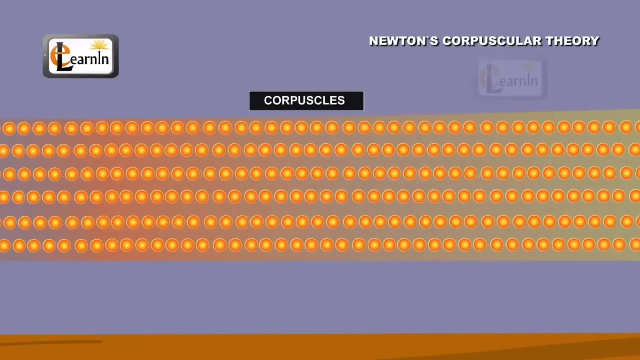 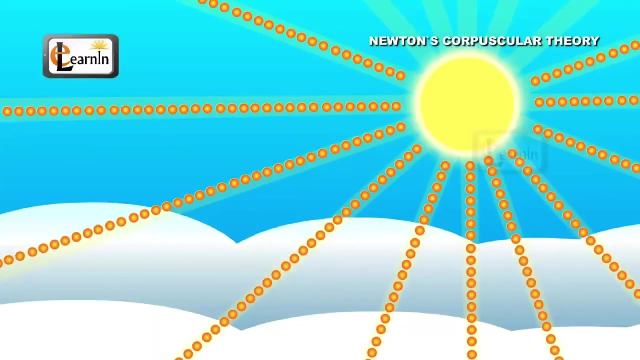 the ice. Here is a short clip that may help you to better understand Newton's corpuscle theory of light. Newton's corpuscular theory of light states the following: Light consists of corpuscles, which are a stream of discrete, tiny light and perfectly elastic particles. Every luminous source, like the 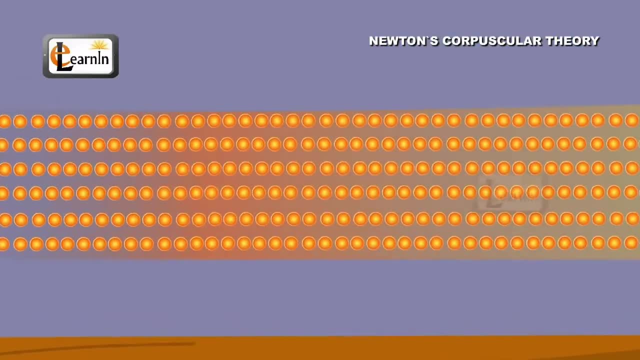 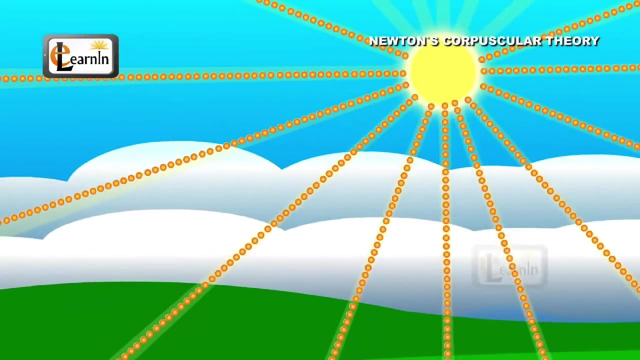 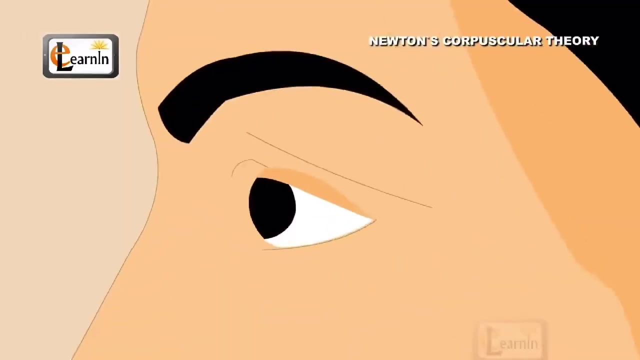 sun, a lamp or a candle emits these corpuscles. These corpuscles travel in straight lines in all possible directions. The rate at which these corpuscles travel may differ depending on the medium in which they disperse. The vision of human beings is a consequence of these corpuscles. 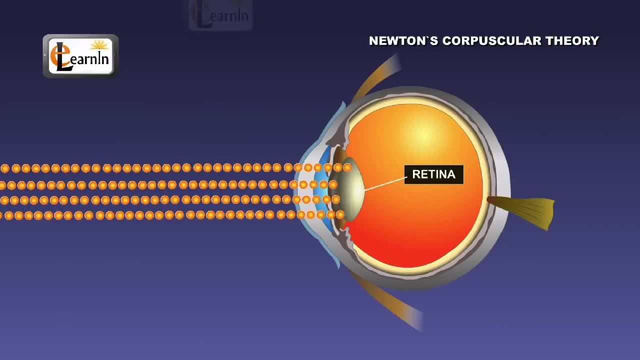 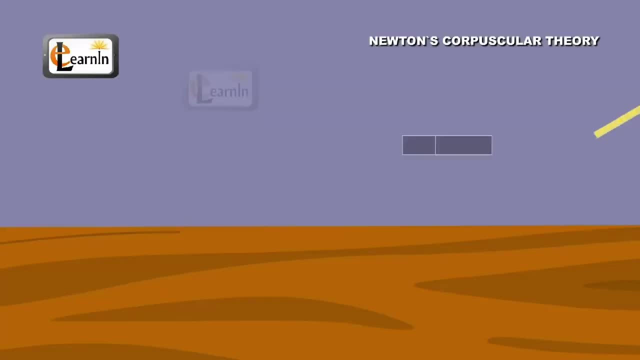 falling on the retina of the eyes. Various colors of light are due to the difference in sizes of these corpuscles. These corpuscles could perfectly explain the concepts of reflection and refraction of light. The reflection of light, which consists of corpuscles, is just like the reflection of a. 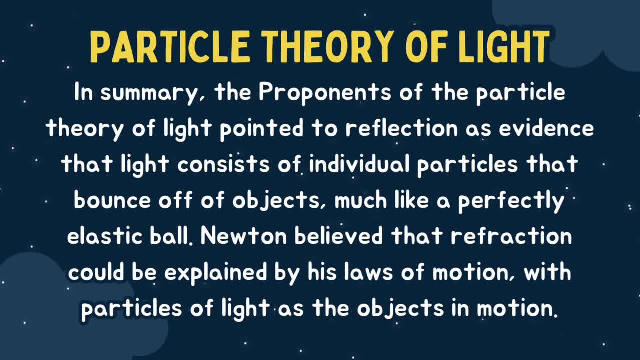 perfectly elastic ball. In summary, the proponents of the particle theory of light pointed to reflection as evidence that light consists of individual particles that bounce off objects, much like a perfectly elastic ball. Newton believed that refraction could be explained by his laws of motion. 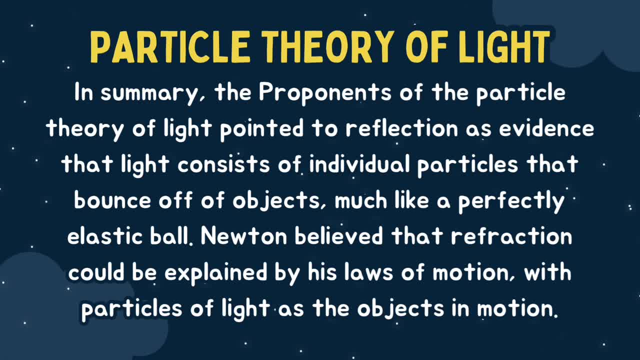 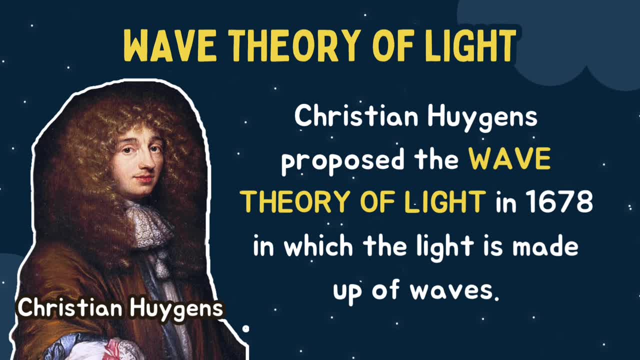 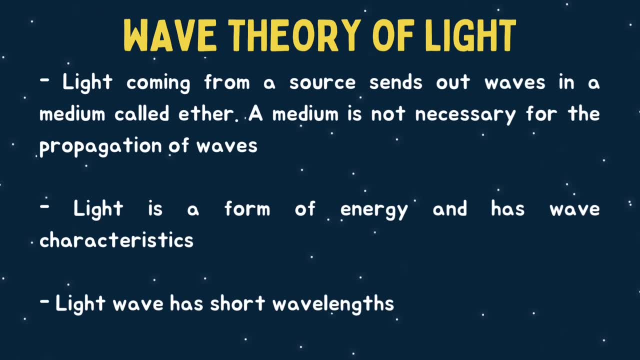 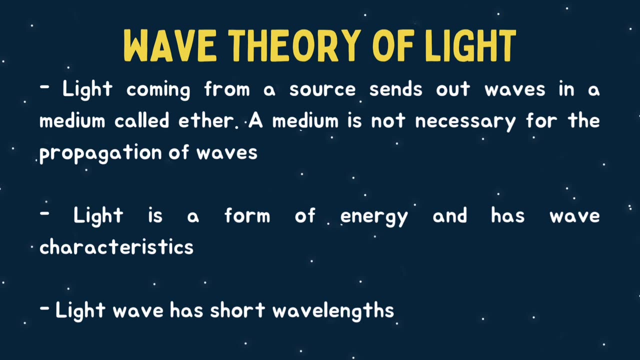 with particles of light as the object in motion. The wave theory of light was proposed by Christian Huygens in 1678, which states that light is made up of waves. Huygens assumed the following concept in his wave theory of light. First, light coming from a source sends out waves in a medium called ether. 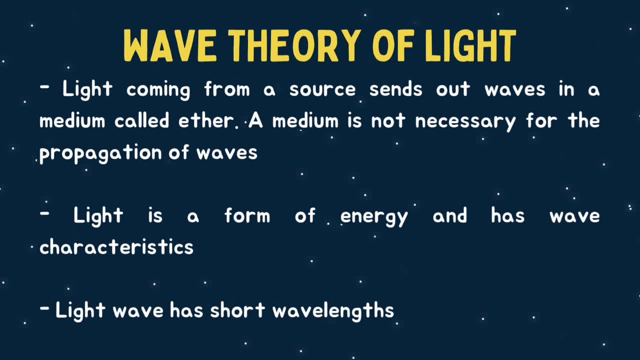 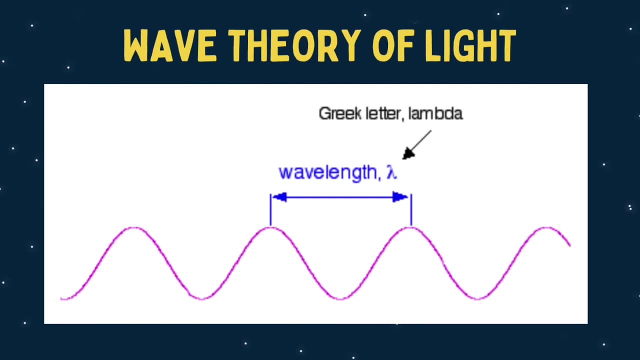 A medium is not necessary for the propagation of waves. Second is light is a form of energy and has wave characteristics. And the last one is light wave has short wavelengths. Wavelength: the distance between any two consecutive crests or troughs is known as wavelength of the wave. 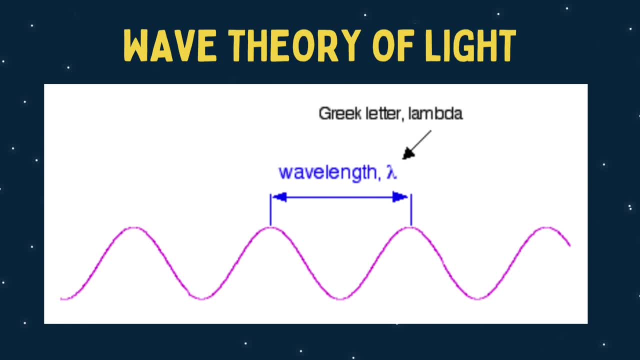 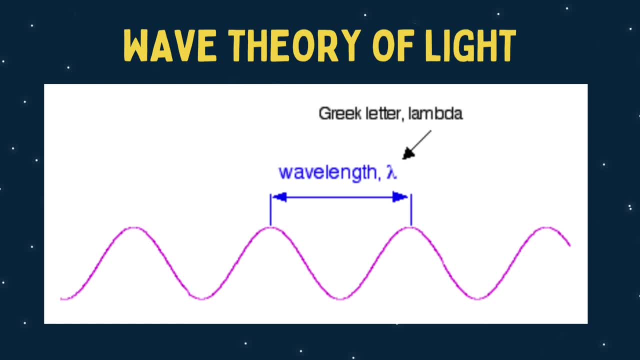 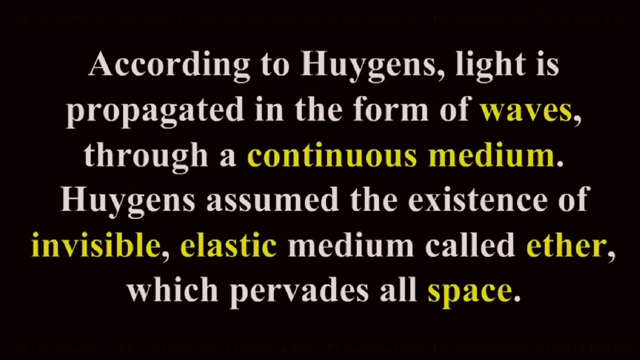 Here is a short video that may help us to further understand the concept of wavelength Huygens' Wave Theory. According to Huygens, light is propagated in the form of waves through a continuous medium called ether. Huygens assumed the existence of an invisible, elastic medium called ether, which pervades all space. 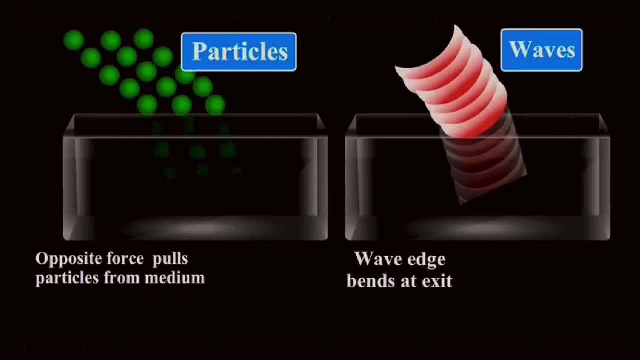 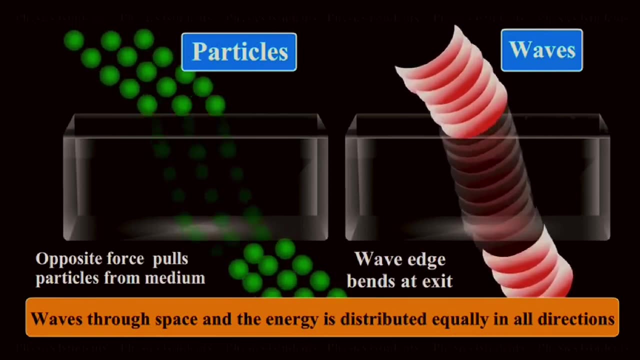 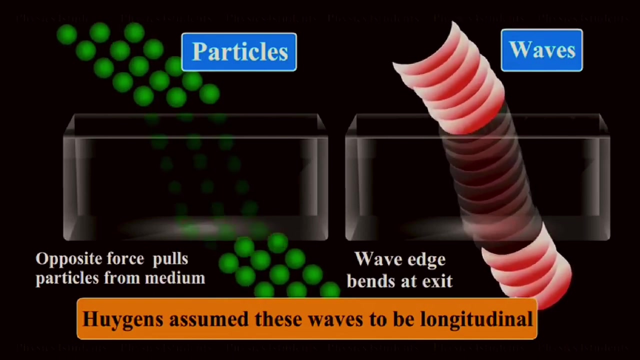 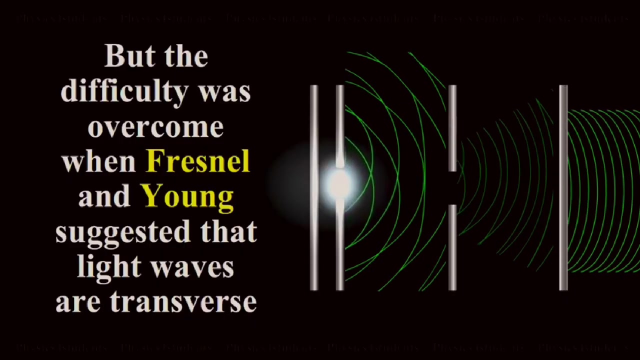 The disturbance from the source is propagated in the form of waves through space and is distributed equally in all directions. Huygens assumed that these waves, to be longitudinal. Initially rectilinear propagation of light could not be explained. But the difficulty was overcome when Fresnel and Young suggested that light waves are transverse. 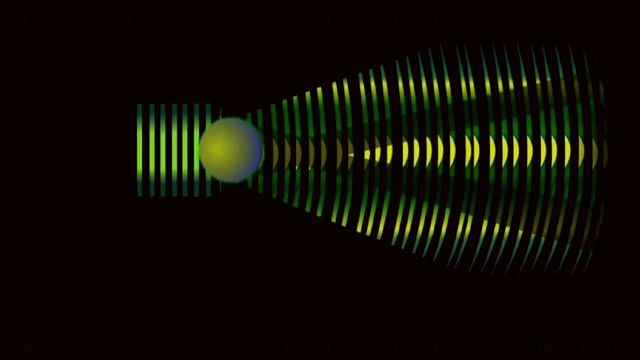 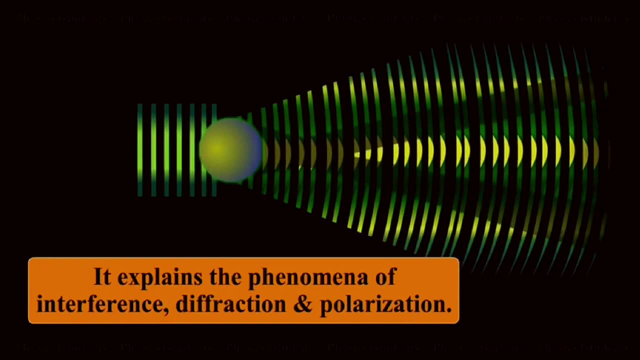 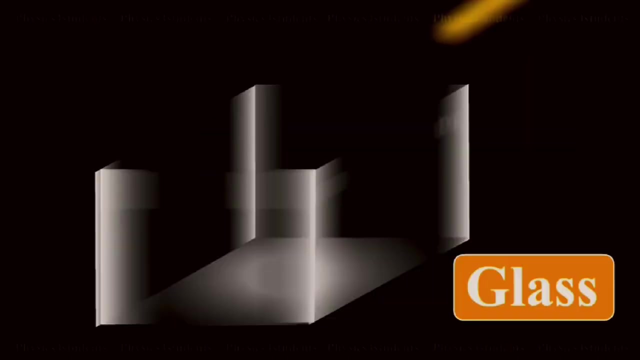 The wave theory could satisfactorily explain all the basic properties and in addition it explains the phenomena of interference, diffraction and polarization. According to Huygens, the velocity of light in a denser medium is less than that in a rarer medium. 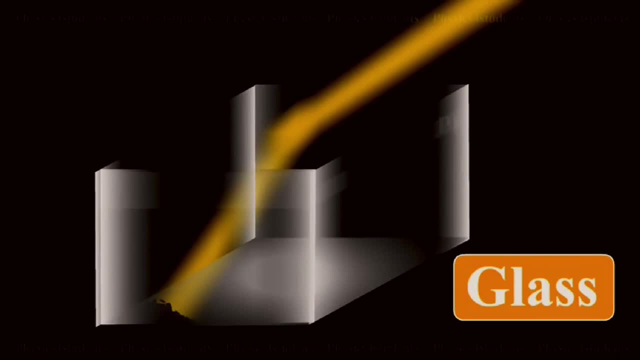 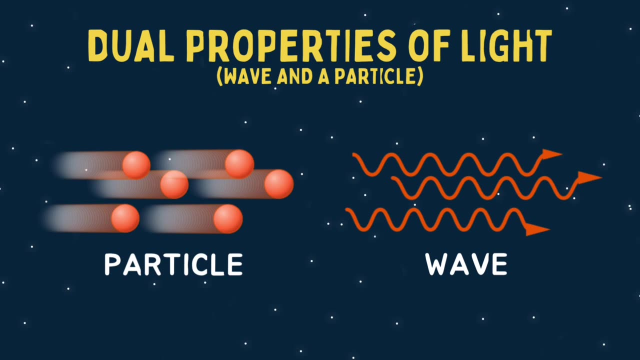 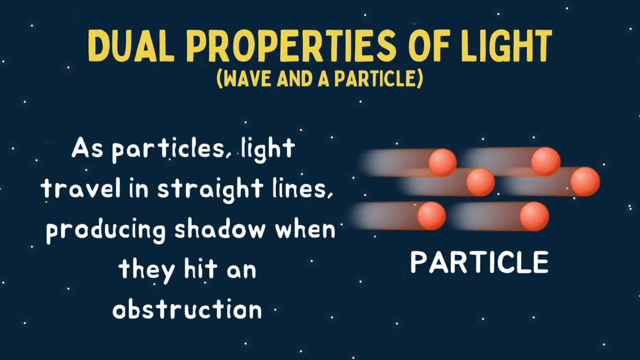 This is in accordance with the experimental result of Foucault. Light can be quite tricky, so let me shed some light on its dual properties. Alright, so here's the deal. When light decided to act like tiny particles, it travels in straight lines. 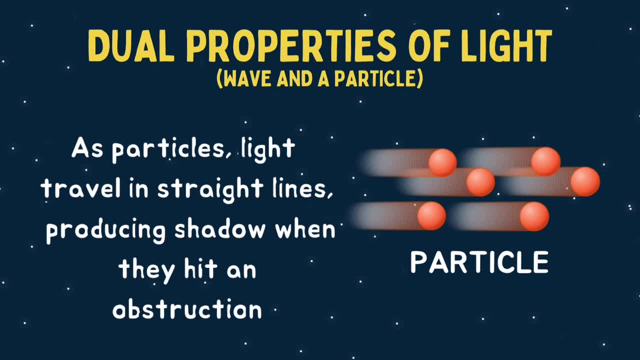 It's like following the road signs, No detours or shortcuts. So when there are obstructions like walls or anything, it produces anemones or shadows. In the image there are tiny particles traveling through it in straight lines. This represents the particle-like behavior of light. 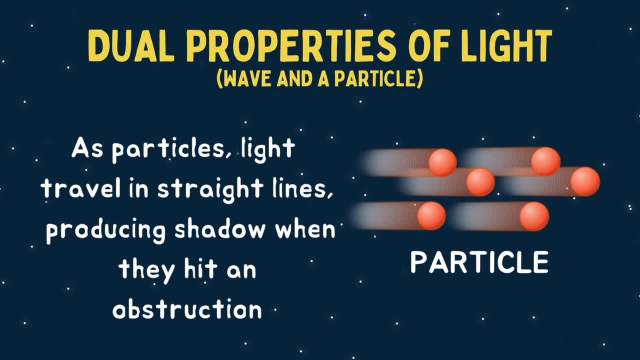 Where light can behave as individual particles called pothons. These pothons travel in straight lines until they interact with an object or surface. The straight lines of the particles in the image symbolize how light travels in a straight path until it encounters an obstruction or gets reflected, refracted or absorbed by an object. 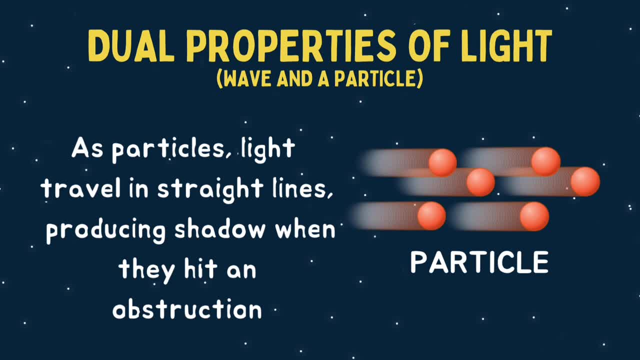 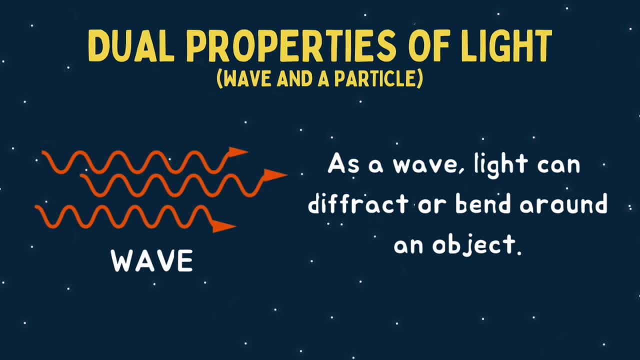 This behavior is a characteristic of light, a characteristic of light as a particle. Secondly, we have its wave-like behavior. It's like a bubble that spreads Light, can travel in waves, just like when you throw a stone in a calm light. 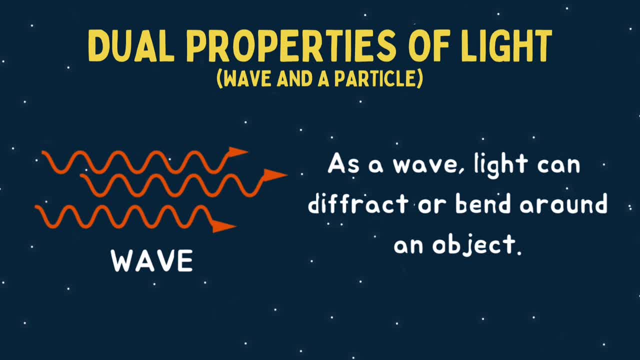 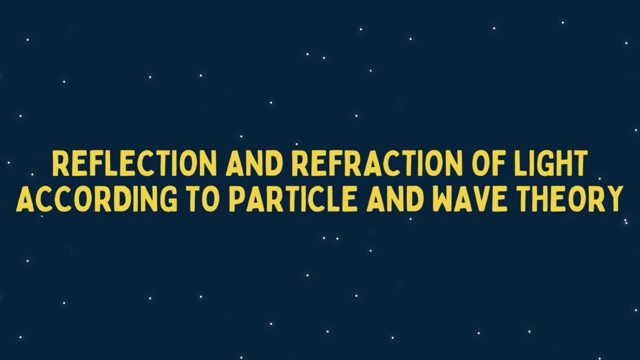 And you see those ripples. It can bend, diffract and interfere with other waves. In other words, it behaves like a smooth wave moving through space. So let's move on to the reflection and refraction of light according to particle and wave theory. 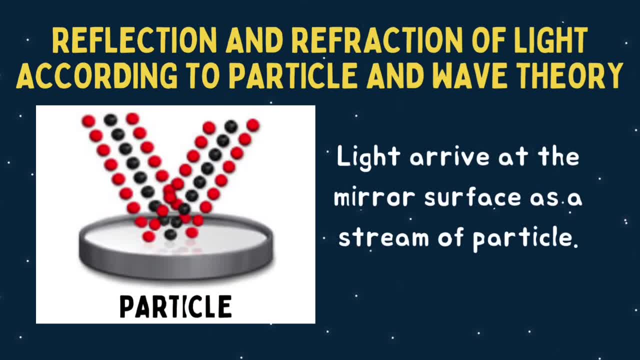 Light arrives at the surface of the glass as a stream of particles, So the case for the particle nature of light is far is longer with respect to the reflection and phenomenon, than refraction. So the light that comes out of a cloud, no matter how close or far, 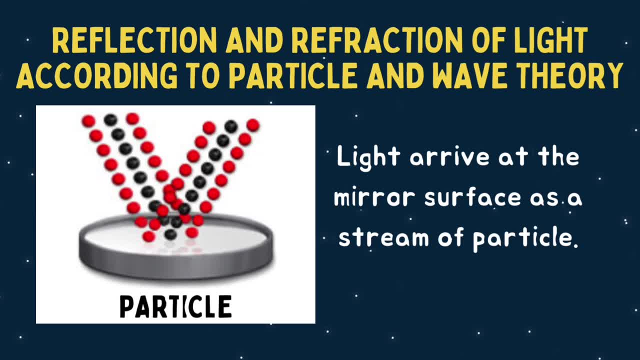 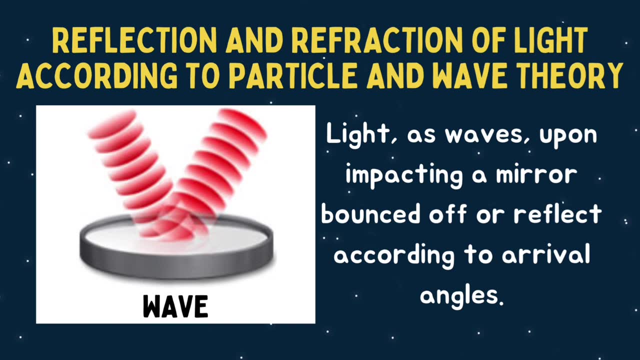 is reflected on the surface of the glass as a stream of particles which bounce off or are reflected from the smooth surface. Light as wave upon impacting a mirror, bounce off or reflect according to arrival angles. According to wave-based theories, the light waves spread out from the surface in all directions and upon striking a mirror. 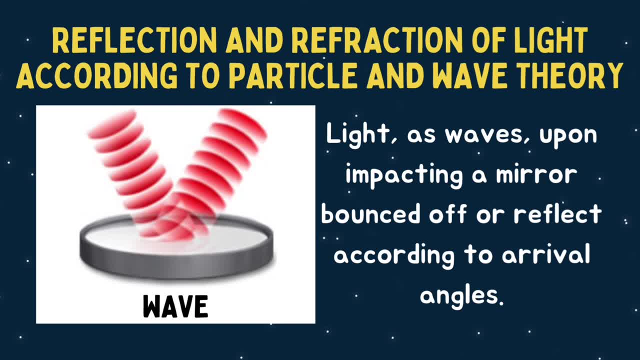 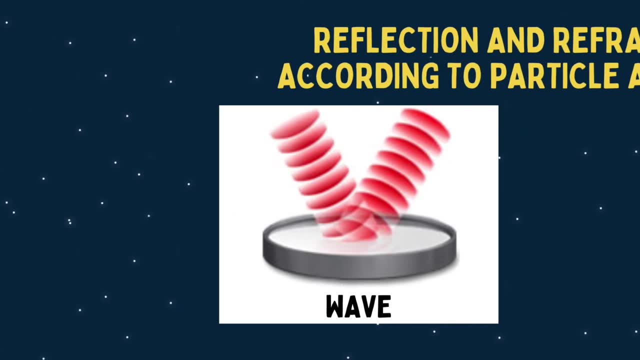 are reflected at an angular distance. This is determined by the angle at which the light arrives. The reflection process is reversed every time it returns to the front. That is why a reversed image follows Light as wave changes direction upon passing from first medium to second medium. 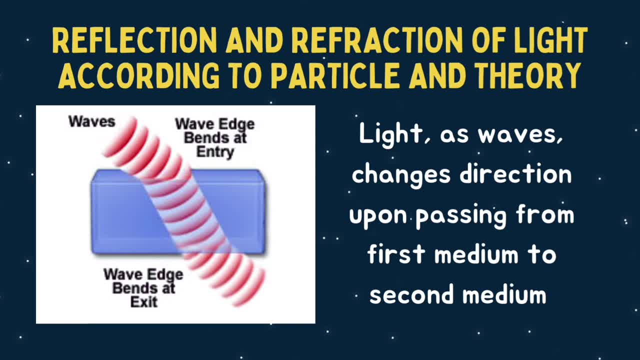 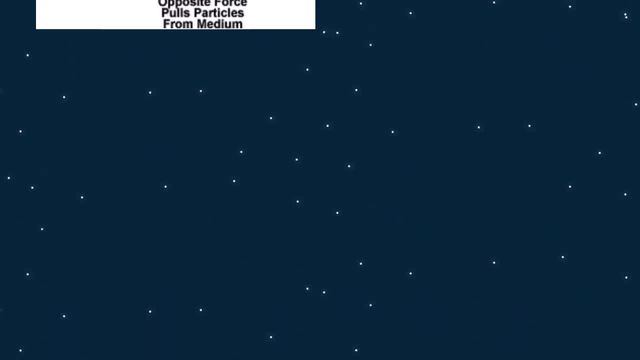 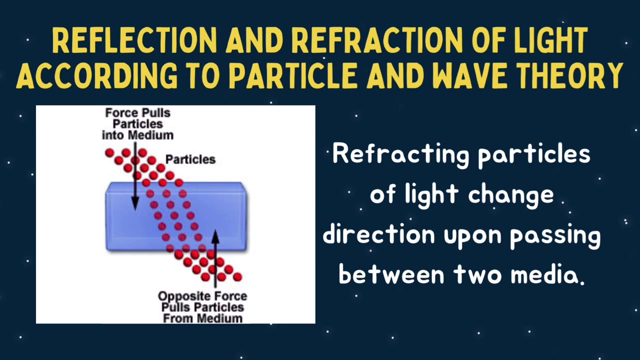 Refraction is the bending of the path of a light wave as it passes from one medium into second medium. The refraction occurs at the boundary and it is caused by a change in the speed of the light wave upon crossing the boundary. So let's move on to the refracting particles of light change direction upon passing between two media. 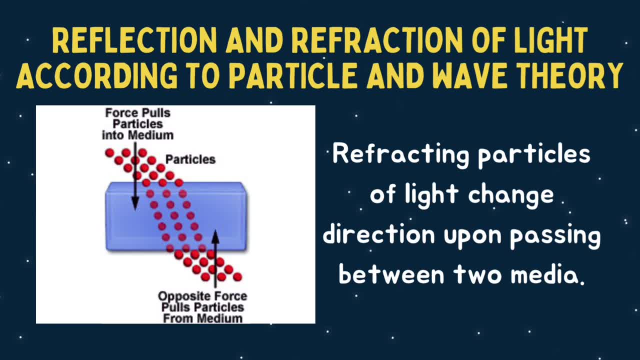 When a beam of light travels between two media having different refractive indices, the beam undergoes refracting and change direction When it passes from the first medium into the second medium. So to determine if the beam of light is formed by waves and particles. 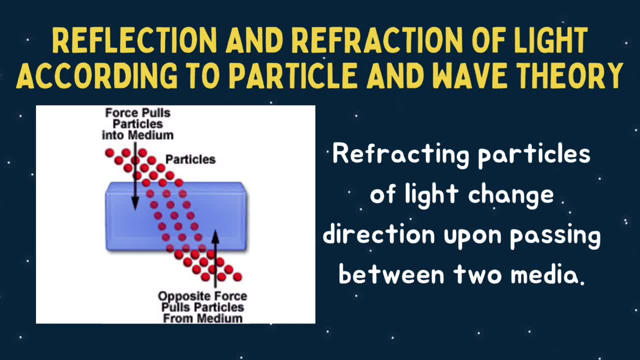 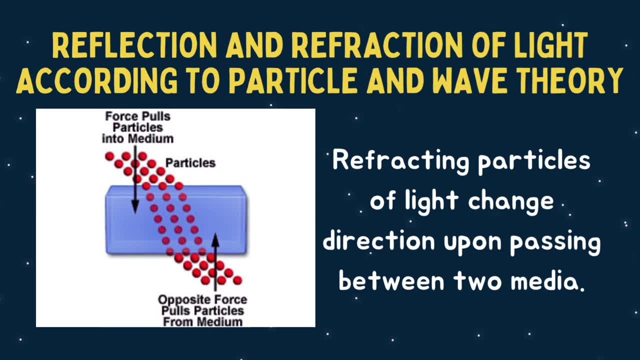 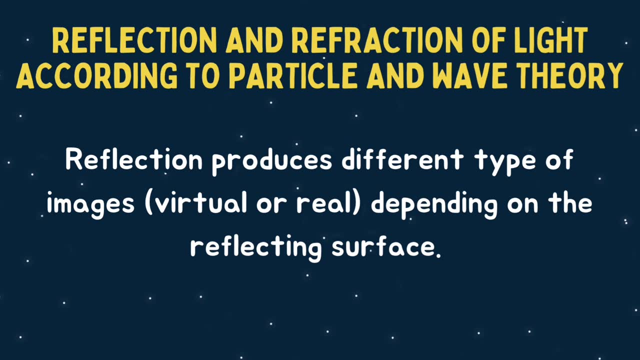 there is a model for each of them that we can use to explain the phenomenon. So next is: Reflection produces different type of image, virtual or real, depending on the reflecting surface. Real images are formed when light rays, after reflection or refraction, converge at a point before a mirror or lens. 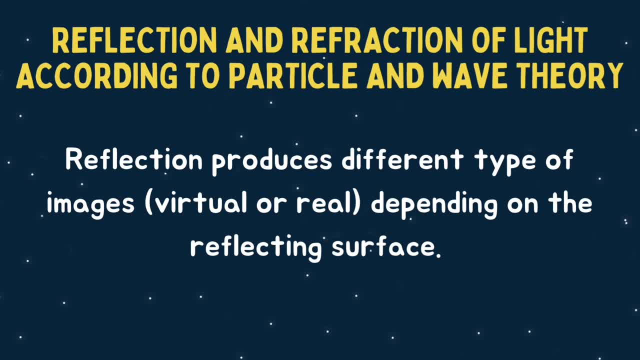 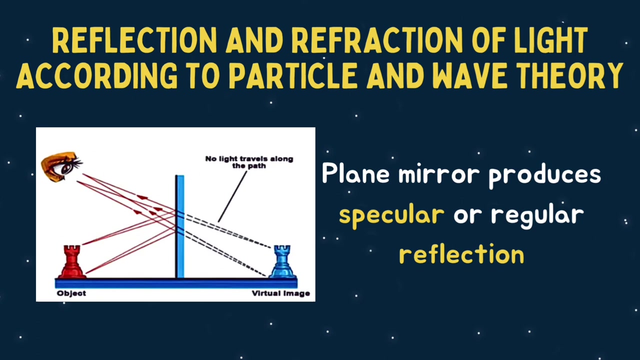 While a virtual image is formed by a beam of light, it changes after reflection and refraction. And about the real image? Real image appears on the screen as a again spiritual image that will never appear on the screen. Plain mirror produces specular or regular reflection. 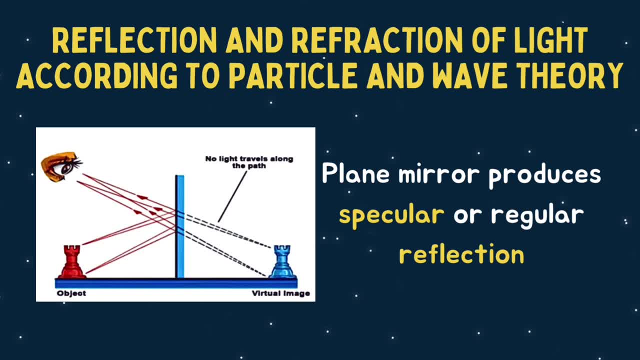 In this case, the light rays are reflected from a smooth, shiny or polished surface, like that of a mirror, and are reflected by a definite angle. Dito yung incident: ray at reflected ray ay gumagawa ng parehong angulo na normal. 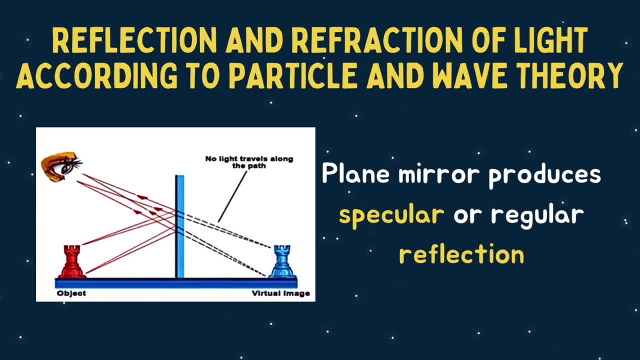 Then yung pagbuo ng isang image ay dahil sa regular na reflection. The image distance and object distance in the mirror are equal. For plain mirrors the object distance is equal to the image distance, That is, the image is the same distance behind the mirror as the object is in the front of the mirror. 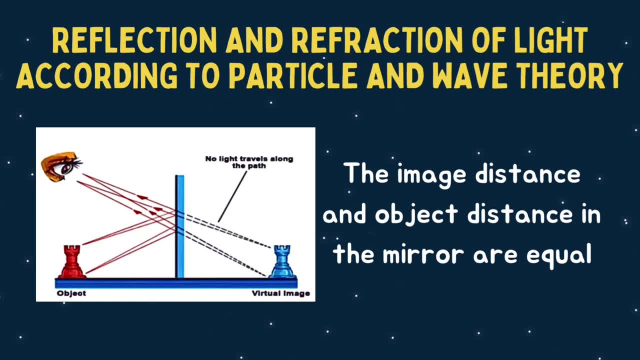 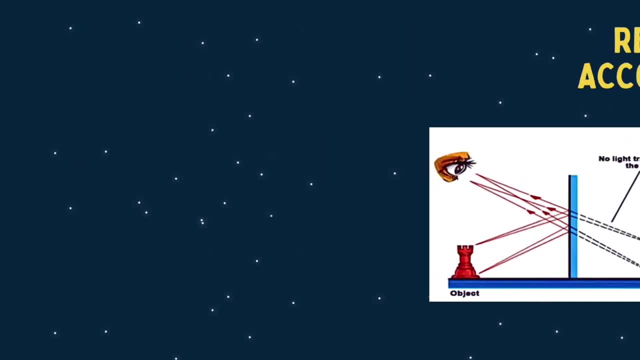 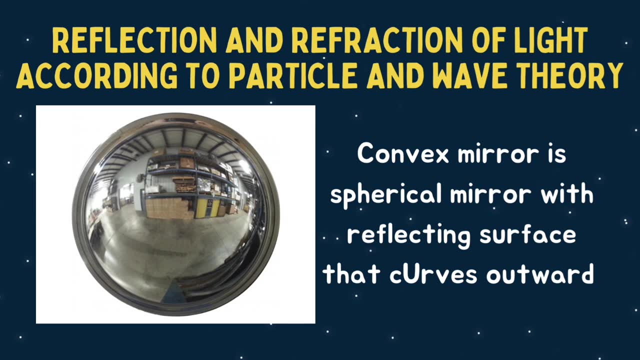 If you stand a distance of 2 meters from a plain mirror, you must look at the location 2 meters behind the mirrors in order to view your image. Convex mirror is a spherical mirror with a reflecting surface that curves outward. The convex mirror has a reflection. 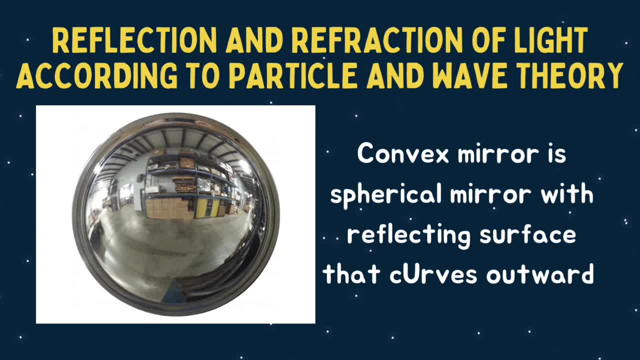 The convex mirror has a reflecting surface that curves outward, resembling a portion of the outside of a ball or a sphere. Lightways parallel to the optical axis are reflected from the surface in the manner that diverge from the focal point, which is behind the mirror. 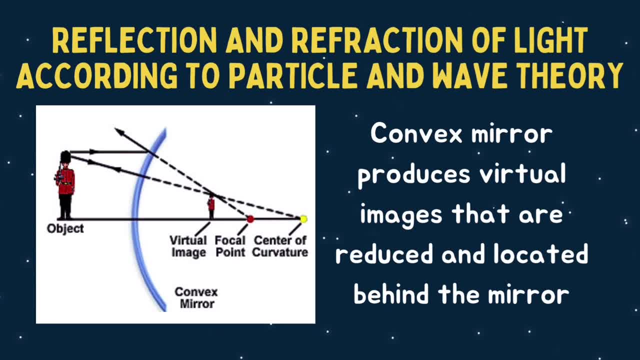 Convex mirror produce virtual image that are reduced and located behind the mirror. Convex mirrors produce virtual image that are located somewhere behind the mirror. It is considered a virtual image because light does not actually pass to the image location. Lumilitaw lamang na dahil sa pagpapakita ng liwanag na nag-iiba mula sa virtual virtual location image. 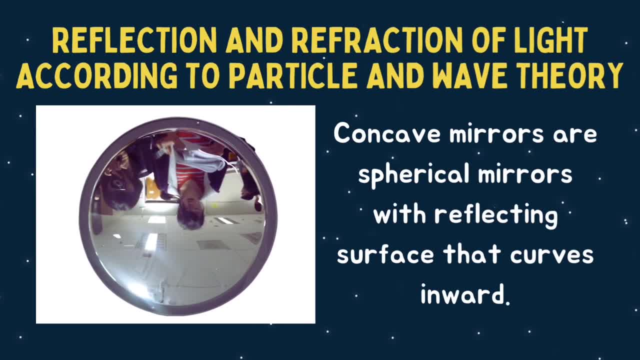 Concave mirrors are spherical mirrors with reflecting surface that curves outward. Convex mirrors produce virtual image that are reduced and located behind the mirror. It is considered a virtual image because light does not actually pass to the image location. It is also considered a virtual image on the surface drive of the object to serve as a Evil tho. 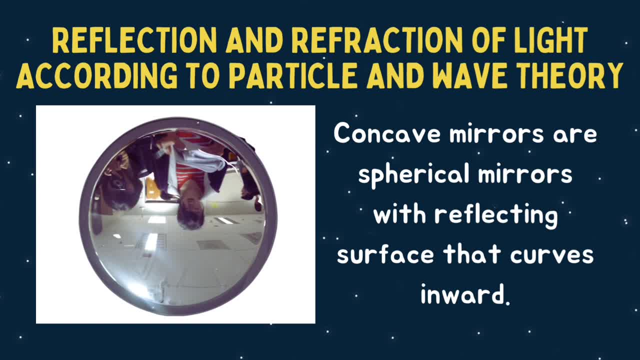 A Concave Mirror has a reflecting surface that curves inward. A concave mirror has a reflecting surface that curves inward away from the incident light. Concave Mirrors reflect light inward to one focal point. They are used to converge light, Unlike convex mirror. 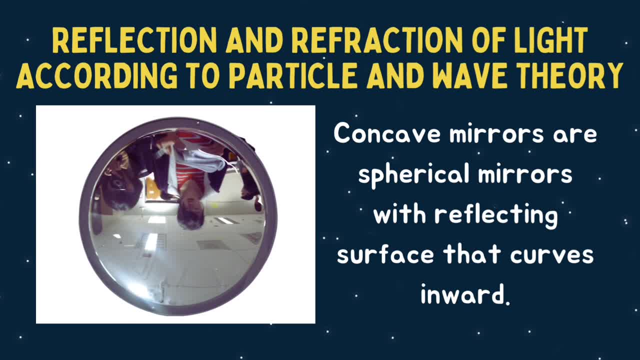 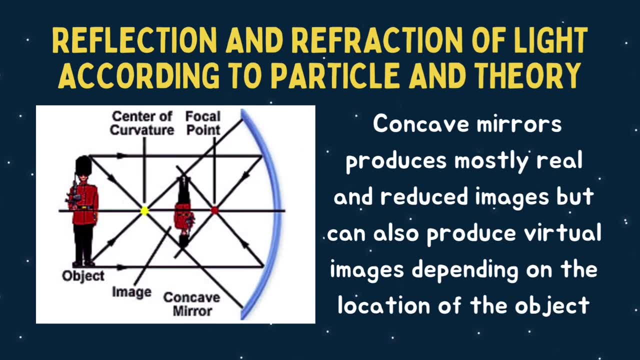 Concave mirrors show different image type depending on the distance between the object and the mirror. Concave mirrors produce mostly real and reduced images, but the sadly very rare worlds are shown as a curve. Concave mirrors produce mostly real and reduced images, but the sadly very rare worlds are shown as a curve. 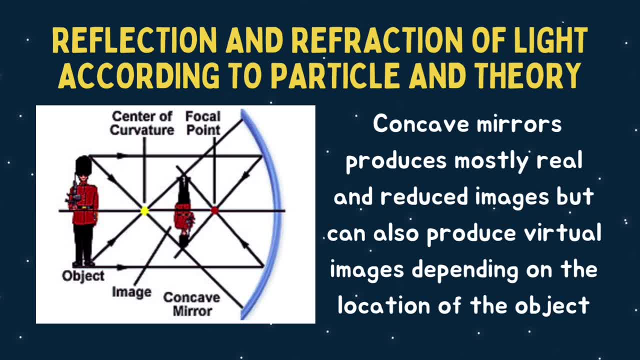 can also produce virtual image depending on the location of the object. So the real image are produced when the object is located a distance greater than one focal length from the mirror. A virtual image is formed if the object is located less than one focal length from the. 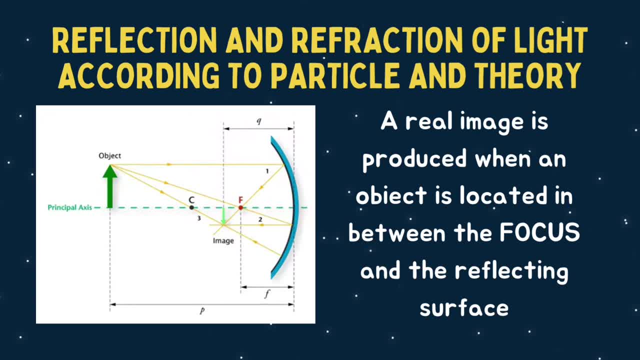 concave mirror. A real image is produced when an object is located in between the focus and reflecting surface. When an object is placed in between the center of curvature and focus, the real image is formed behind the center of curvature. The size of the image is larger than that of the object. 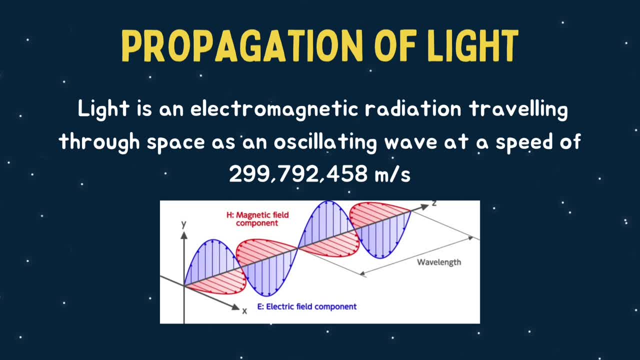 Propagation of light is the process by which an electromagnetic wave circulates, Transfer energy from one point to another, is referred to as a light propagation To understand the propagation of electromagnetic wave. electromagnetic waves are created as a result of vibration produced between an electric field and magnetic field. 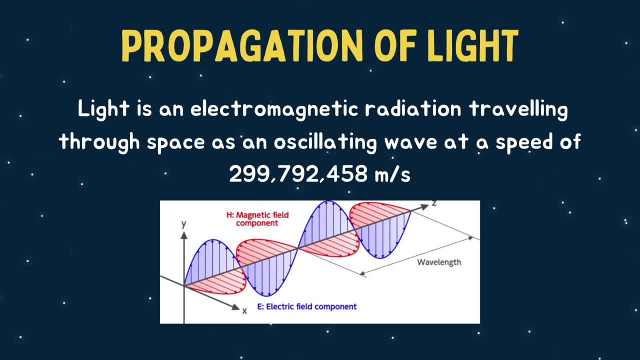 In simple words, electromagnetic waves emit an accelerating electrical charge. These waves have the types of traveling and magnetic transfer waves. This wave is oscillating or vibrating, so this wave has both the magnetic and the electric field component, and this is traveling at a speed of 299,792,458 meter per second. 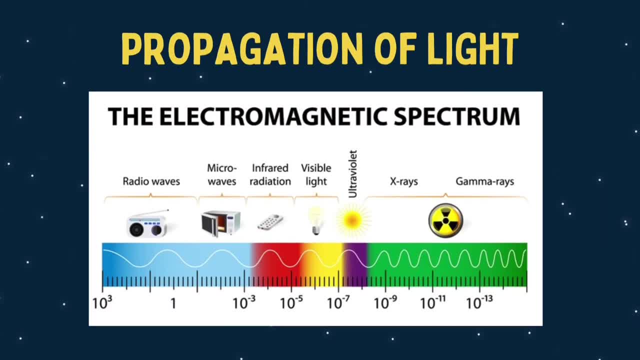 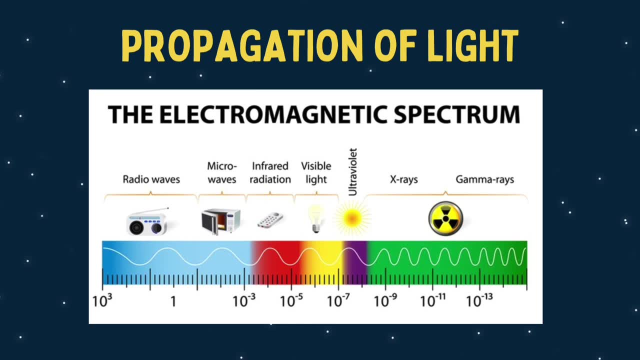 in the vacuum of space. Aside from this, different electromagnetic waves are formed in the electromagnetic spectrum. This shows the frequency and wavelength ranges. This shows the frequency and wavelength ranges. This shows the frequency and wavelength ranges of electromagnetic waves. The electromagnetic spectrum is formed by radio waves, microwaves, infrared visible light. 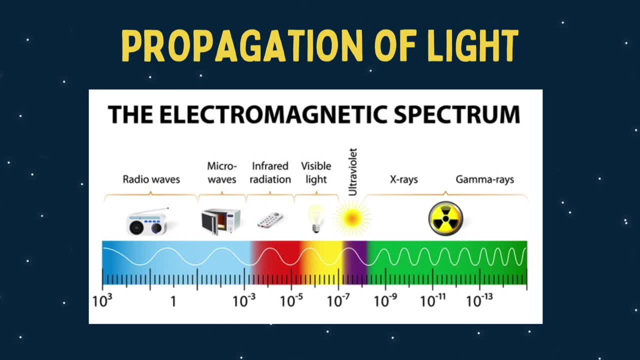 ultraviolet x-ray and gamma rays, which we often use for communication, medical treatment, diagnosis and scientific observation. It is important to remember that radio waves are the lowest frequency wavelength and the gamma rays have the lowest wavelength. However, the gamma rays have the highest frequency. 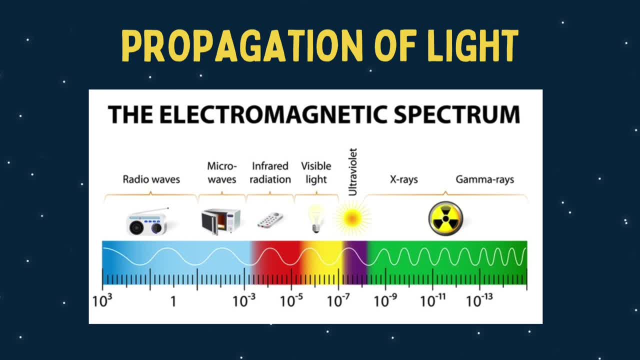 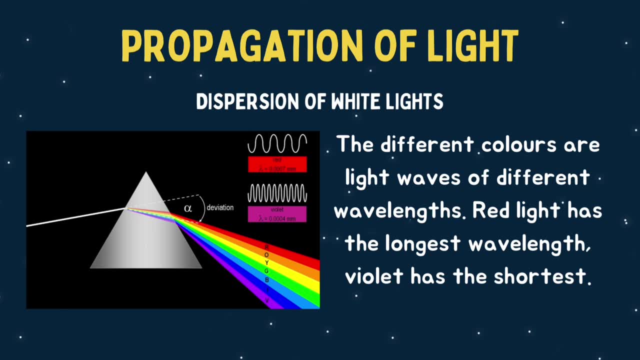 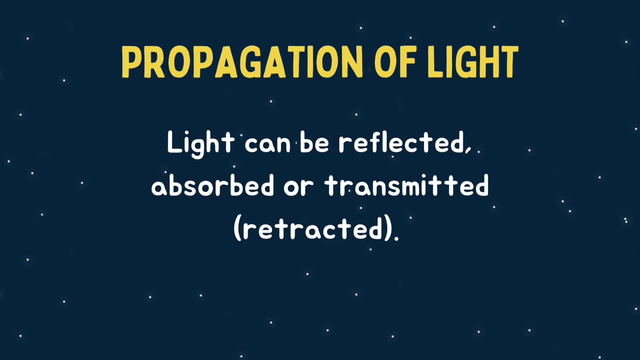 energy, and the radio waves have the lowest frequency energy in all magnetic waves. Next is dispersion. This is the separation of the components of visible light in the spectrum. This is because of the difference in their degrees or refraction. Light can be absorbed or transmitted. 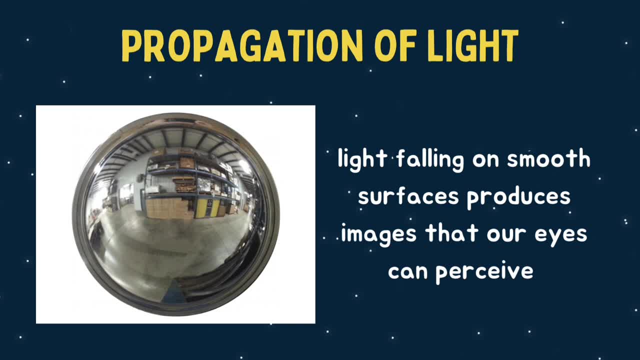 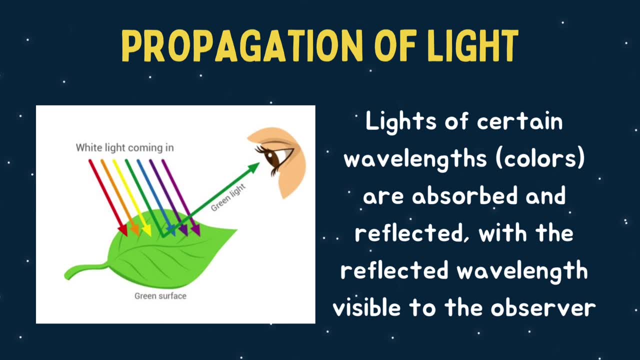 When light falling on smooth surface, it produce image that our eyes can perceive. We recognize the color due to the observation in the reflection of light's certain wavelength or colors. If seeing an object of white, that means all the colors are reflected. If we are seeing a black object, that means that all the